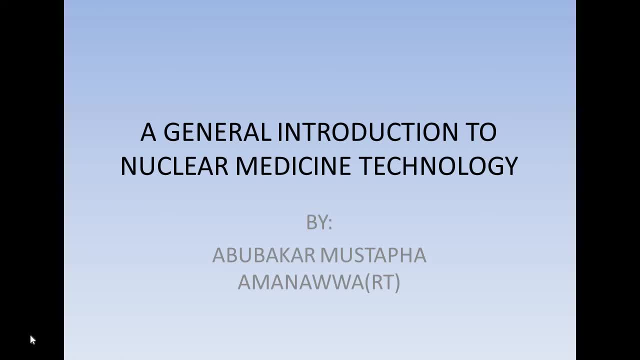 Assalamu alaikum, Good day to you all. My name is Abu Bakar Mustafa Amanawa, a radio imaging technologist. To give you a general introduction on the course nuclear medicine technology, there will be a series of videos. This is just the beginning. This is just a general introduction about the nuclear medicine technology. There will be a series of videos. Please stay tuned with us at this channel of physics of radiology. If you have not subscribed to our channel, please subscribe to our channel. 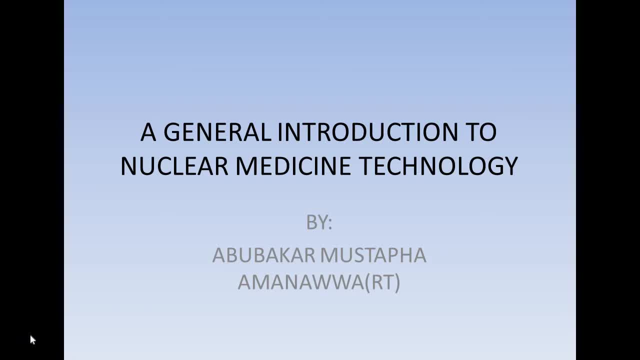 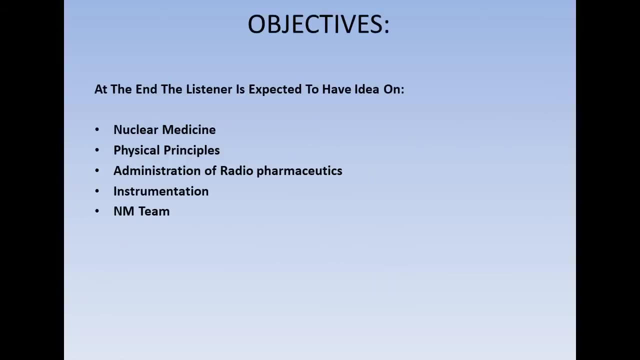 Please subscribe and hit the like icon and click on also the bell icon so that whenever we upload our videos you will be seeing them. Okay, the objectives of our today's lecture is that at the end of this, the listener is expected to have an idea on nuclear medicine. That is, what is the nuclear medicine? Also, the listener is expected to know the physical principles of. 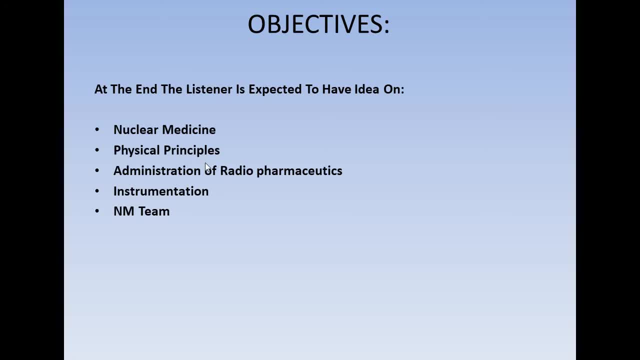 this nuclear medicine? What are the physical principles of this nuclear medicine? Also, the listener is expected to know about the administration of radio pharmaceutics. How are these radio pharmaceutics administered? There is also instrumentation. The listener is also expected to have a little idea about the 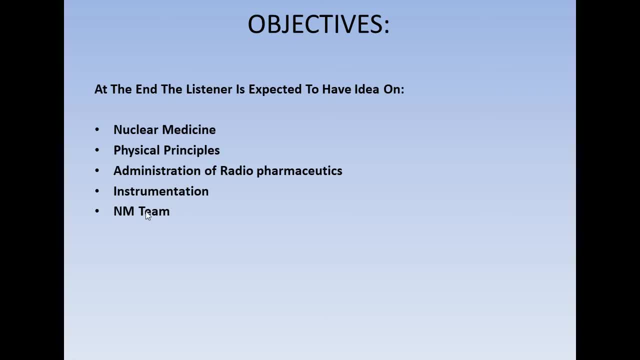 instrumentation of nuclear medicine technology, Although in subsequent videos that will be coming, we will have detailed explanation about all this, But today we will just be having short explanation regarding the same also. lastly, the listener will also get to know about the nuclear medicine team, what, who is involved in nuclear medicine? 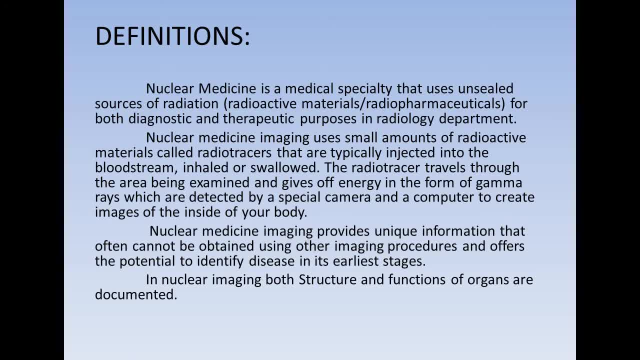 what is this nuclear medicine? nuclear medicine is nothing but a medical speciality that uses unsealed sources of radiation, that is, the. it uses radioactive materials or radio pharmaceuticals for both diagnostic and therapeutic purposes, and radiology department, nuclear medicine imaging, uses small amount of radioactive materials, called radio traces, that are 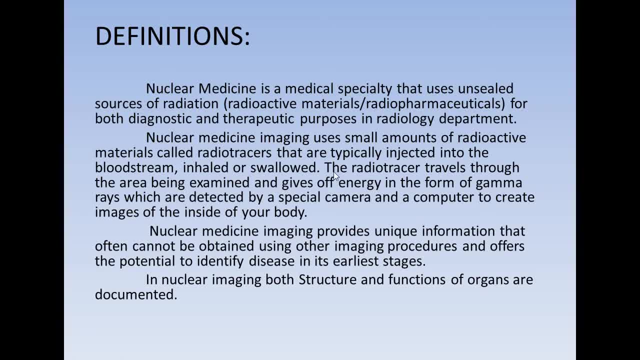 typically injected into bloodstreams, inhaled or swallowed. this means that nuclear medicine technology or imaging uses small amount of radioactive materials. this small amount of radioactive materials that are used by nuclear medicine- they are called radio, radio traces, which are typically they can be injected, inhaled or swallowed. if they are injected, they are injected directly to 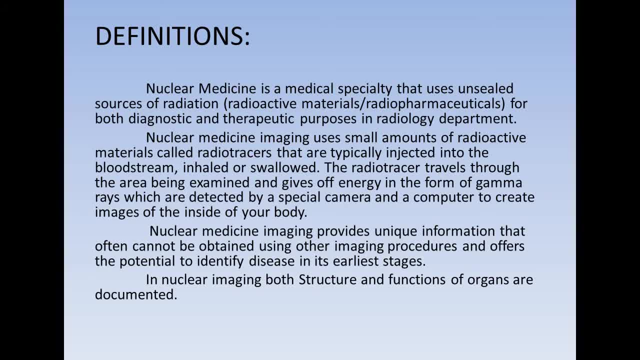 the bloodstream and, while inhaled- and also they can be swallowed, the radio traces travels through the area that is been examined. this radio traces, when they are swallowed, injected or inhaled, they travel directly through the area that is been examined and when they travel through this area, they will give up an energy in the form. 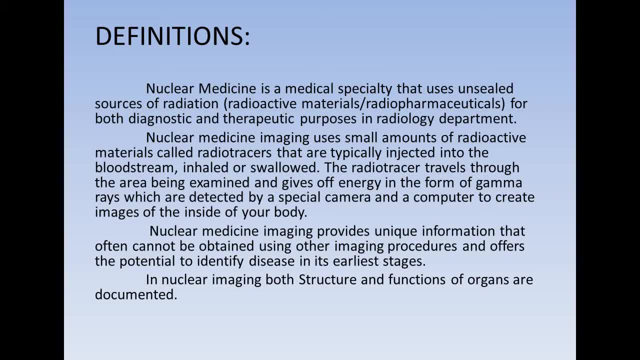 of gamma rays which are detected by a special camera and this gamma ray that is been released by this. radio traces in the area been examined. they have been detected by a special camera and a computer to create images of inside of your body. this is a brief about the nuclear medicine technology. also, we can 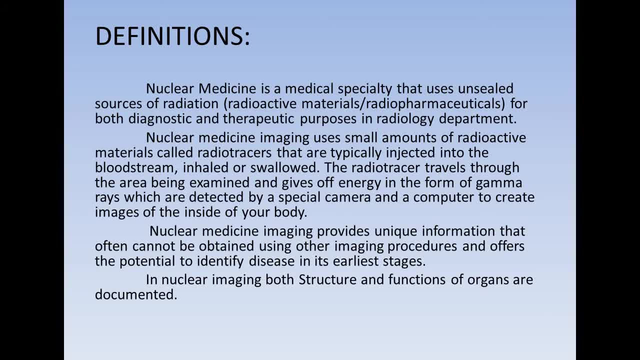 see that nuclear medicine imaging programs are very well known in the- provides unique information that often cannot be obtained using other imaging procedures, and offers the potential to identify diseases in their earlier stages. As part of the advantage of this nuclear medicine, it can be used to detect diseases at their 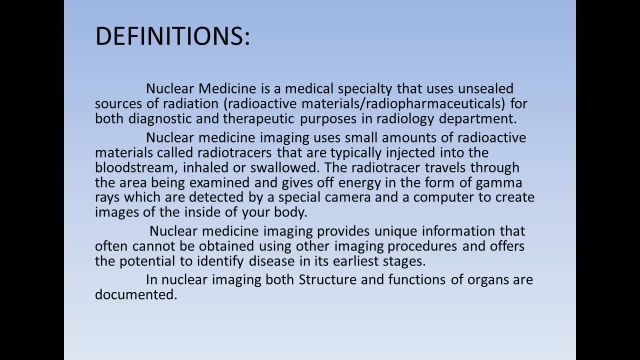 earliest stages In nuclear medicine. also, you get to know that imaging can be both structural and that of functions of organs. What this statement means is that the statements in nuclear imaging, both structural and functions of organs, are documented. This means that, if you recall, from a plane X-ray you can only see the structures, but 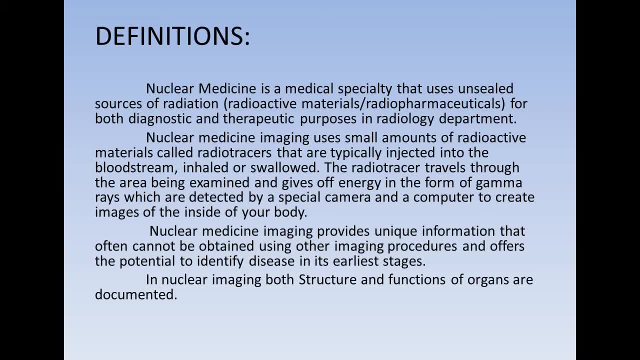 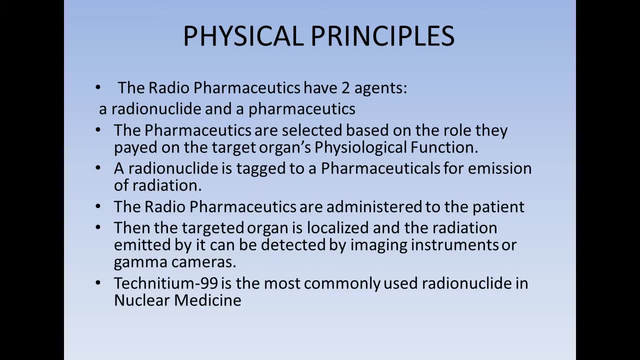 the functions are not visible, but here, in nuclear medicine technology, even the functions are documented or can be observed or seen While performing the procedure. What are the physical principles of this nuclear medicine? The basic principle of the physical principle of this nuclear medicine is that it uses radiopharmaceutics. 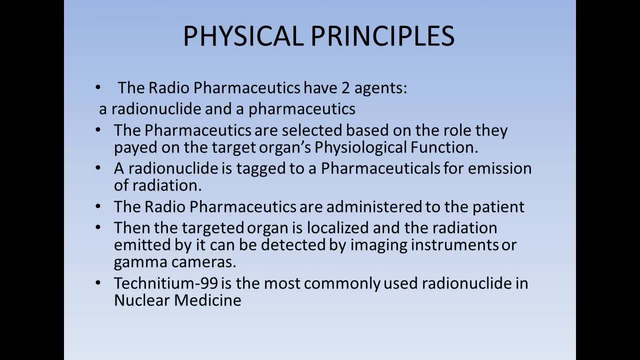 and this radiopharmaceutics have two agents, that is, a radionuclide and a pharmaceutics. Talking about the pharmaceutics, the pharmaceutics are selected based on the role they played on the target physiological function. This means that 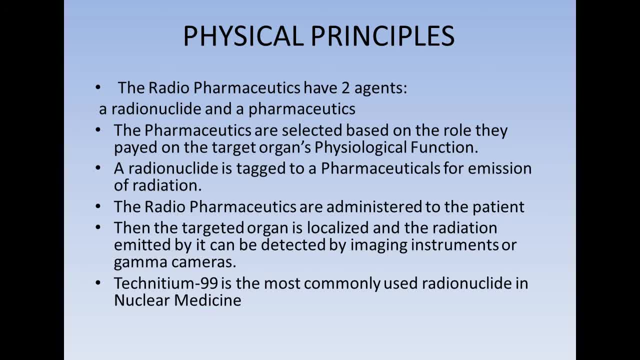 If we have a pharmaceutics that can work on a specific organ, then we will get to know about the physiology. Then we will use that pharmaceutics and attach it with a radionuclide for that so that there will be emission of irradiation using that pharmaceutics. 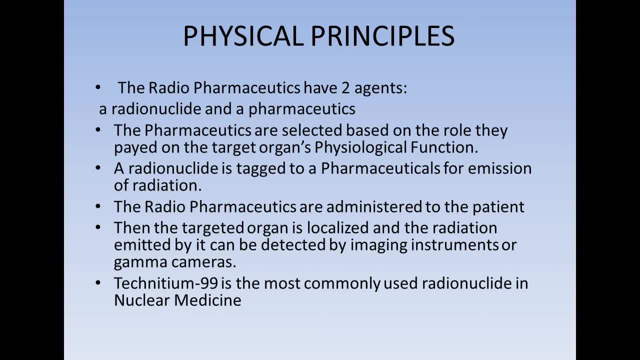 Combining this pharmaceutics and the radionuclide will give us what is known as radiopharmaceutics, and this radiopharmaceutics and this radiopharmaceutics are administered to the patients. Then, when they are administered to the patients, they will target an organ. 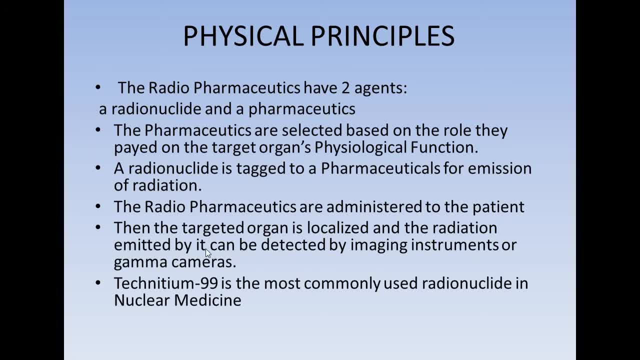 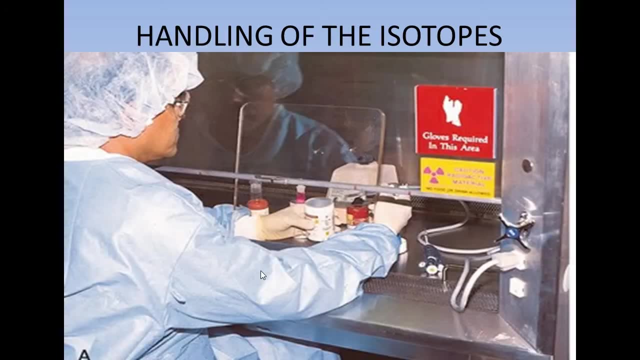 That is to say, the target organ is localized and the radiation emitted can be detected by imaging instruments, or what we call the camera. This is the most commonly used radionuclide in nuclear medicine. That is the technician 99.. if you look at this image- and this is just a short explanation or a diagram that will tell. 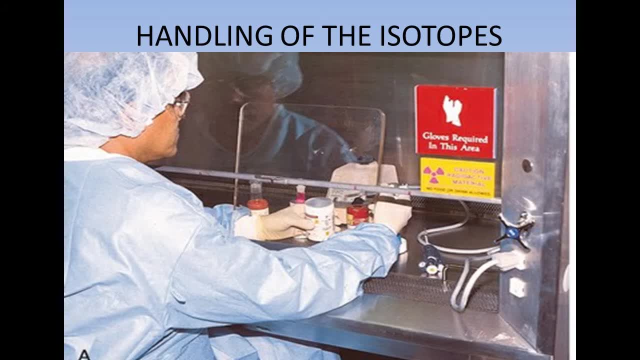 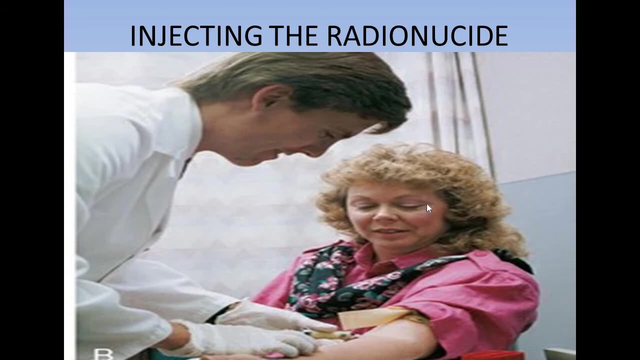 you about how these isotopes are handled. you can see the technician or the technologist using his, having his gloves and with led apron so that to avoid the radiation. to avoid radiation, those also here. this is image of technologies injecting a new clade to the patient, using as 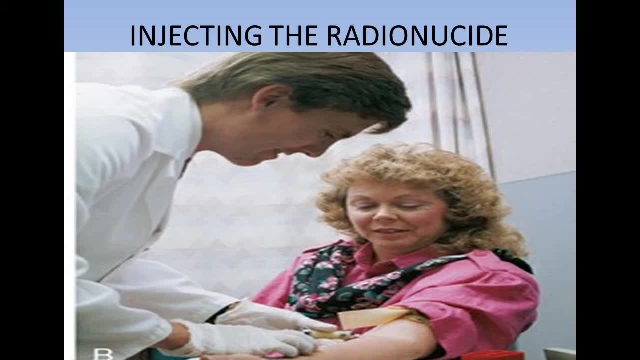 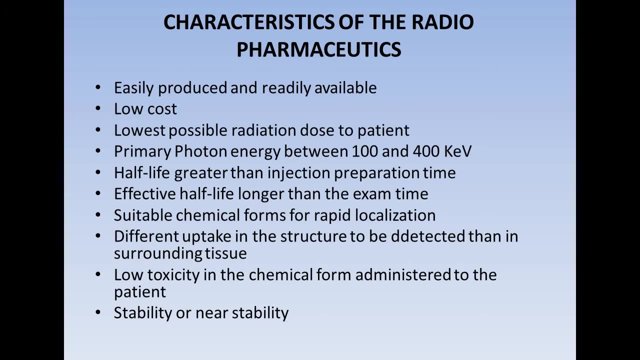 range, and this range is also having to avoid irradiation of unwanted parts and to reduce the radiation exposure of both the patient and the technologist. Also, we will talk about the characteristics of this radiopharmaceutics, These radiopharmaceutics: what are their characteristics, What are they expected of? 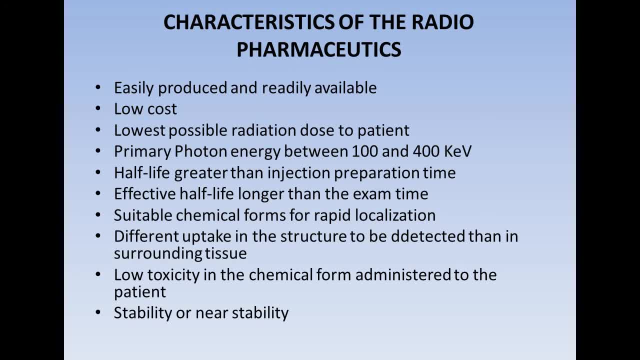 What we expect of a radiopharmaceutics is that it should be easily produced and it should be readily available. It should be of low cost. It should have the lowest possible radiation dose to patients. That is the radiation, If you remember, from Alara. we need the lowest possible. 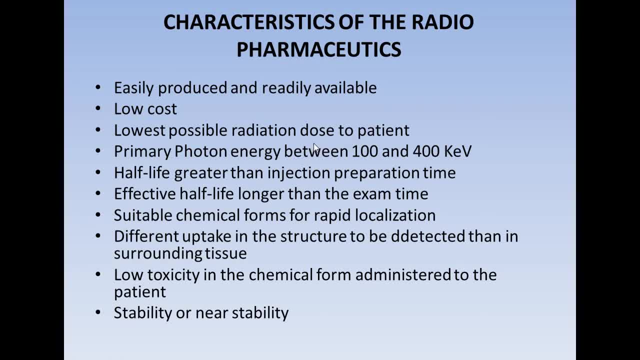 radiation, but the radiation that we give, that will be useful. Alara it means as low as reasonably achievable. That means that there should be low and possible radiation dose to patients, But with meaningful information. Also we will talk about the primary photon energy. 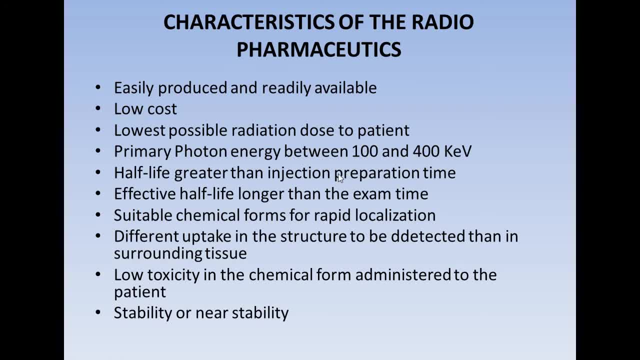 of between 100 and 400 keV is required as a characteristic of the radiopharmaceutics. Also, there is half-life. This half-life should be greater than injection preparation time. We need the half-life to be greater than the injection preparation time so that the radiopharmaceutics 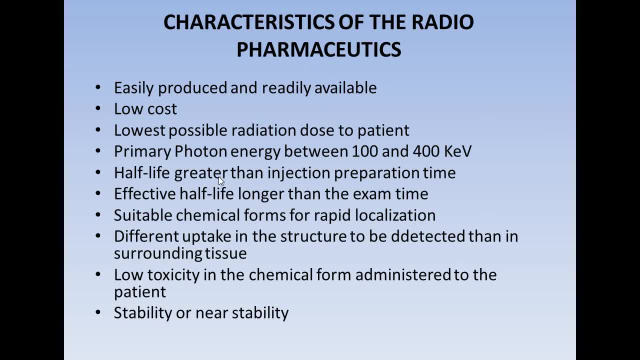 will not exceed its half-life while preparing the injection. The half-life, the effective half-life- longer than the exam time. also, It should be longer than the exam time so that we will be able to complete the exam in case there are any delays during the procedure. Also, it should be suitable. 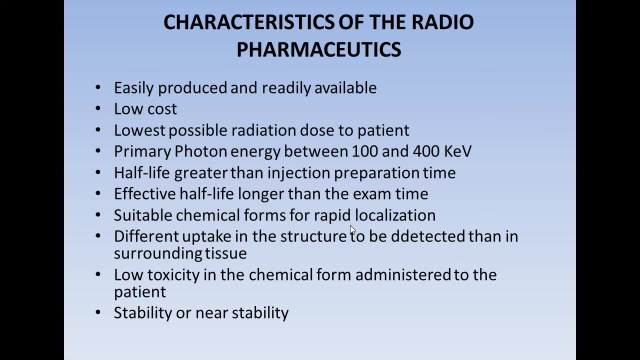 chemical forms for rapid localization, so that it can easily locate where it is Different optics in the structure to be detected than in surrounding tissues. Also, there is low toxicity in the chemical form administered to the patient. We also need the radiopharmaceutics. 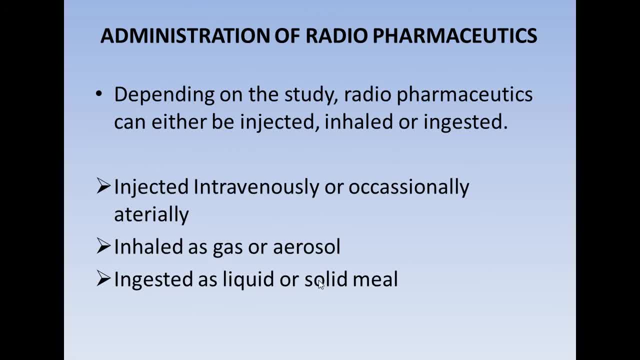 to be stable or nearly stable. How do we administer this radiopharmaceutics? That is, the administration of radiopharmaceutics Depending on the study we are doing. radiopharmaceutics can either be injected, inhale or ingested. it depends on which type of study we are. then what do we want to see, depending? 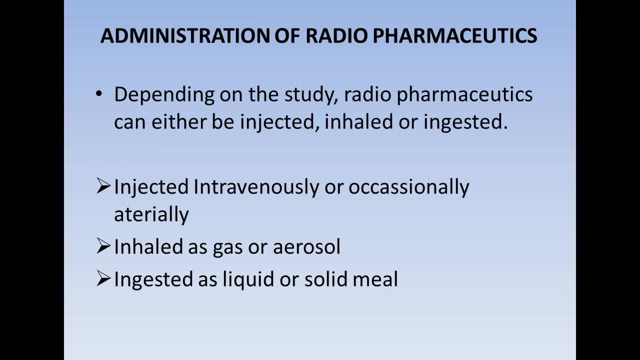 on that. this radio from aesthetics can either be injected. they can either be injected- we can inhale them- and also we can inject, ingest them. when we are talking about injected, we are talking about in the intravenous level, occasionally arterially, and when we are talking about 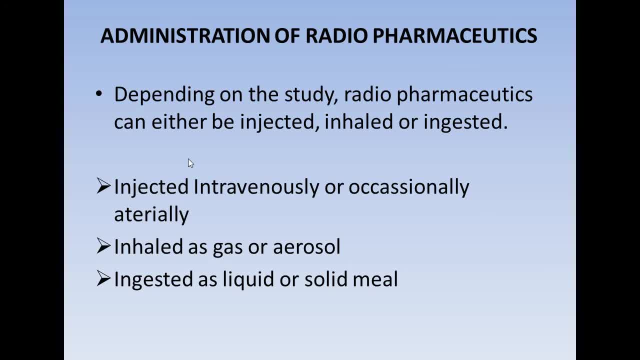 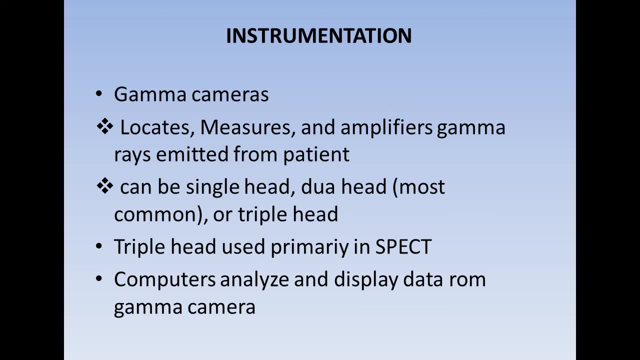 inhalation, that is, as a gospel aerosol. when we are talking about ingested also also we are talking about as liquid or solid milk. what are this instrumentation for? the instrumentation for nuclear medicine technology did the document? the instrumentation is that we are, we have a gamma. 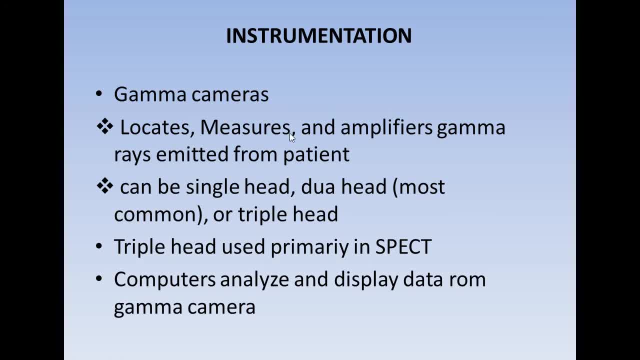 cameras and this, in gamma cameras, indicates, measure and amplify gamma is emitted from a patient, which means that if this radio from the cities are given to the patient and the days emission of gamma rays, this gamma cameras will locate this gamma, this gamma rays that are been emitted by the patient as a result of the radio from aesthetics that was administered to him. they 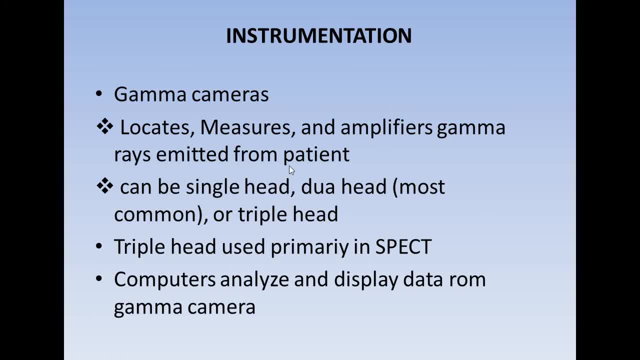 will locate them, measure them and amplify the gamma is emitted from this patient so that they can easily diagnose what is wrong with the patient, and also they can be single head. you, you, you, you, you, you. you need to know that this instruments, that is, the gamma camera. we have a single head gamma. 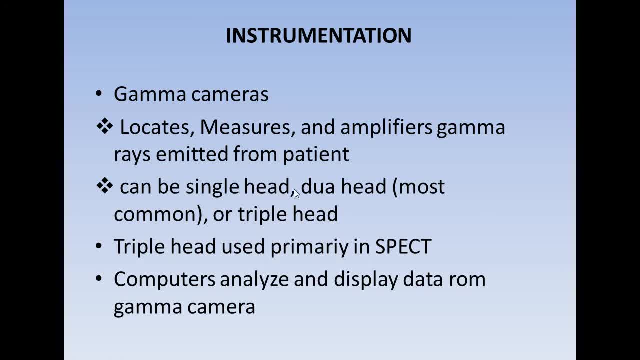 camera and there is dual head, that is to it has two head and it is the most common, that is readily available and the most department or they can even be triple head in the maximum possible capacity camera. triple head is used primarily in aspects, that is, the single positron. 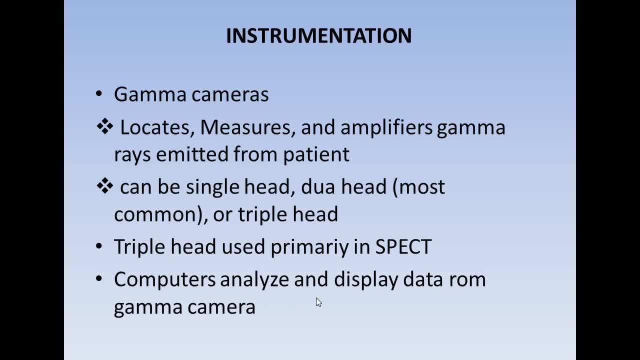 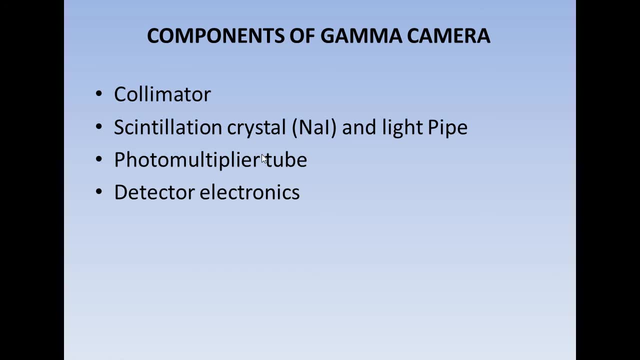 emission: computer tomography. computers analyze and display data from gamma cameras. computers analyze and display data from gamma gamma camera- component of gamma cameras. what are the component of this gamma camera? this gamma camera, as we've discussed, also have its own components and in our subsequent lectures you will get to know about the component of this gamma camera. but for 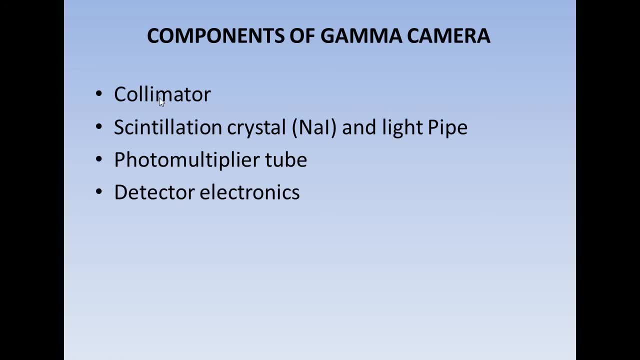 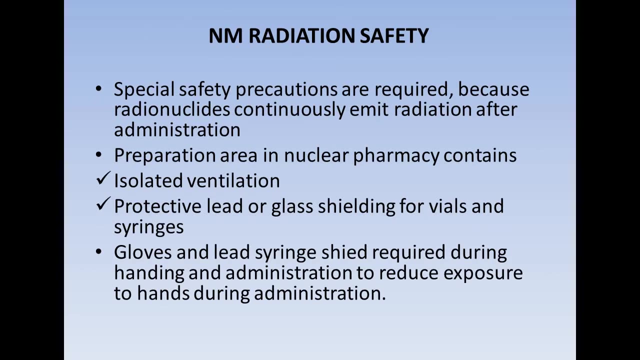 just introductory, for the purpose of introduction. the gamma cameras have collimators, scintillation crystal and the light pipe. it also have a photo multiplier to detect, to electronics. and now to be talking about the nuclear medicine, radiation safety. we know in radiology department radiation safety is always our number. 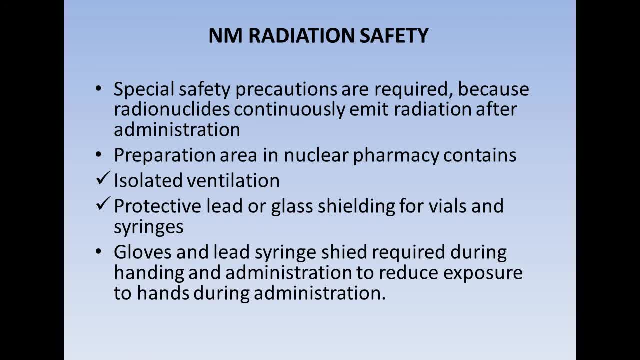 one priority. we will have to care for the patient as well as the technologist, so as to be safe from radiation taking about this nuclear medicine. radiation safety will talk about the special safety precautions are required because radionuclides continuously emit radiation after administration and also. 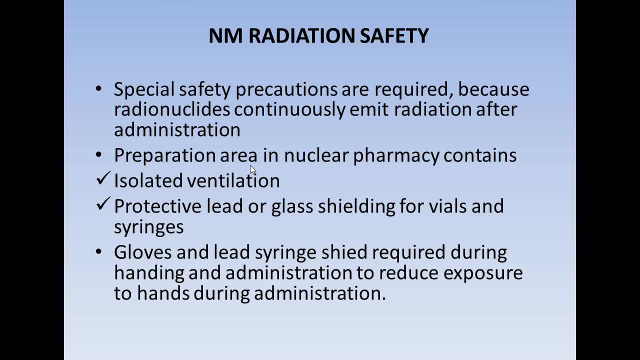 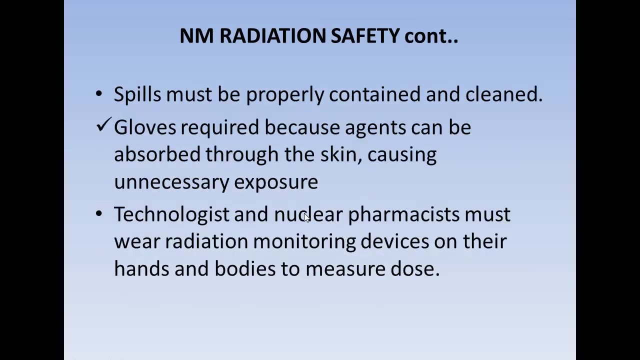 preparation in nuclear pharmacy contains isolated ventilation, protective lid or glass shielding for valves and syringes, gloves and lead syringes shield required during handling and administration to reduce exposure to hands during the administration. this radiation safety of nuclear medicine are straightforward. also, the spills must be properly contained and cleaned, that is. 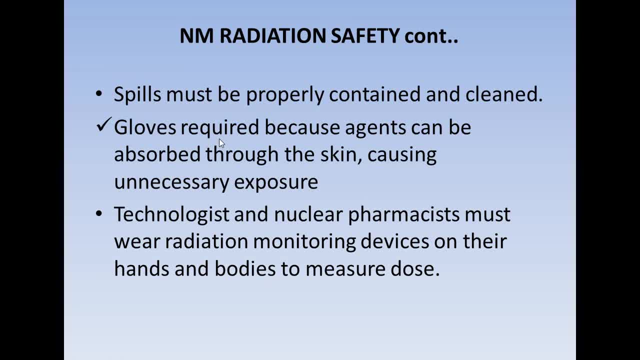 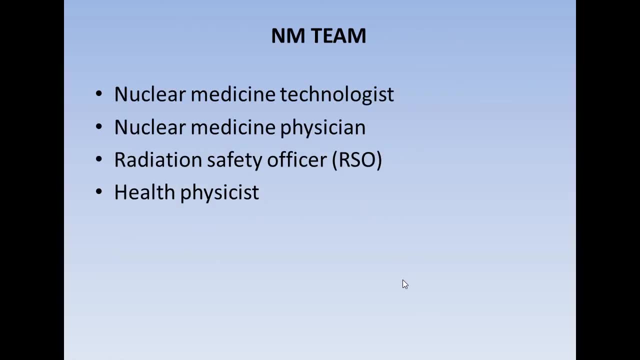 dispelled from radionuclides. globes are required because agent can be absorbed through the skin, causing unnecessary exposure. technologies and nuclear pharmacists must wear radiation monitoring devices on their hands and bodies to measure their dose, so as for them to be safe to know the amount of radiation they are consuming. 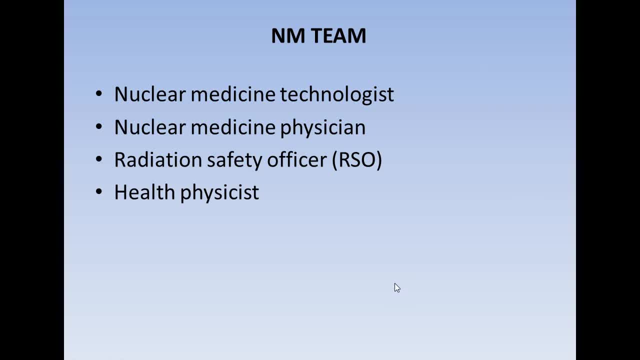 the nuclear medicine technology team. this, uh, there are the- the team of nuclear medicine. nuclear medicine is that we should have a nuclear medicine technologist, that is the person who will be in charge of all the procedures, while the nuclear medicine physician that is, uh, the doctor, uh a radiologist, and also we should have a radiation safety officer. 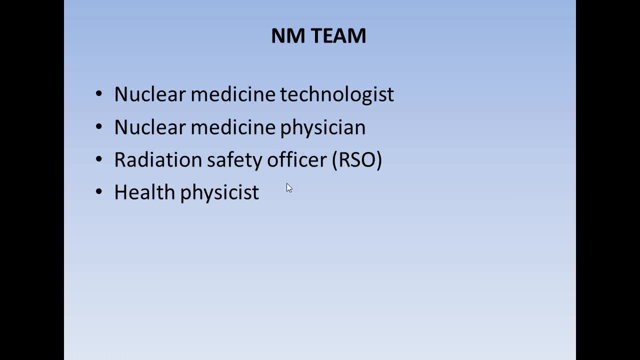 who is in charge of the radiation safety of both the patient, the general public, and the nuclear medicine physician, as well as the nuclear medicine technologist, there should also be a health physicist in the nuclear medicine team. uh, here we come to the end of our today's uh lecture. 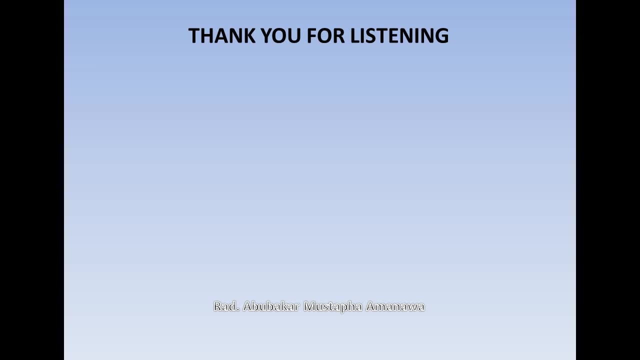 for nuclear medicine technology. and uh, don't forget, i told you it's just a, an introduction of nuclear medicine technology. there will be subsequent uh series of videos regarding the nuclear medicine technology. stay with us. don't forget to hit the bell icon so that whenever we upload new videos, you'll be able to see it. we will notify you and, if you have not subscribed, 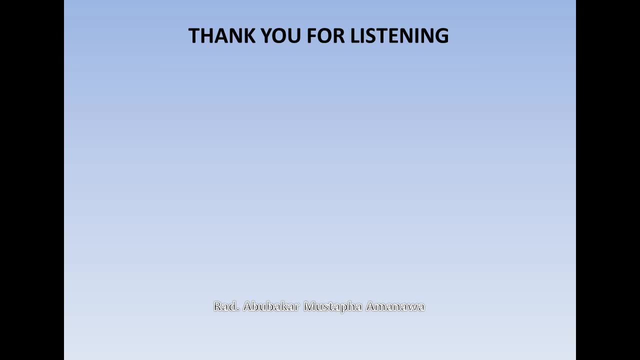 our channel. please do subscribe our channel. physics of radiology. thank you once again. i remember abu bakar mustafa amanawa. thank you.